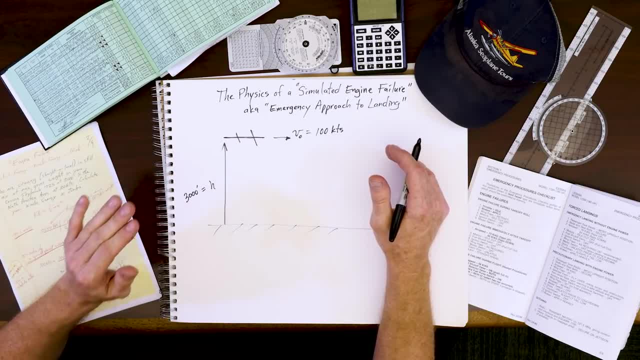 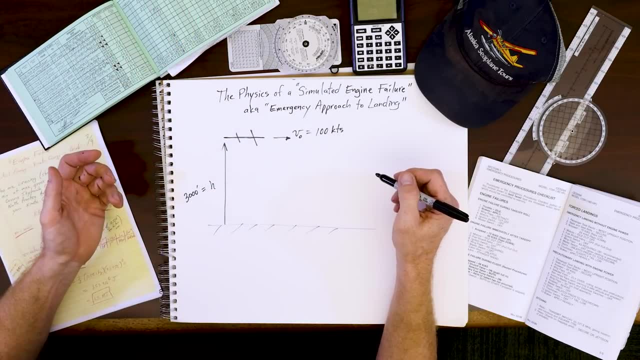 Or they make the field fine, but because they were too high and too fast, they end up with too much kinetic energy and they end up having an accident at the end of the field When they hit the oak tree or something, The oak trees or the barn. 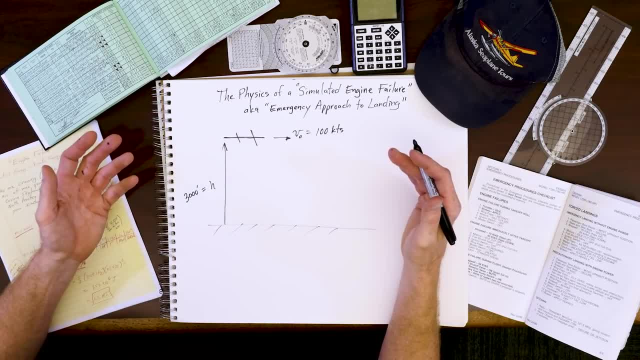 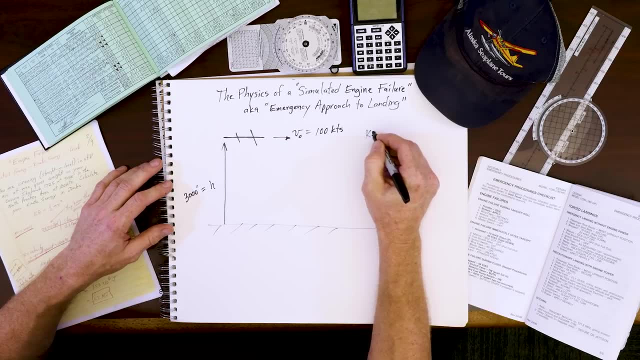 And so I'm going to compare impulse and momentum if they properly get like a wheat field or a cornfield or something. So our first goal here is to get the kinetic energy. Our kinetic energy, as you recall from Physics 103, is one half mass velocity squared. 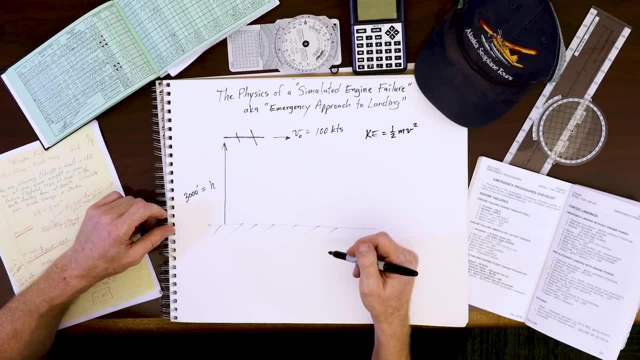 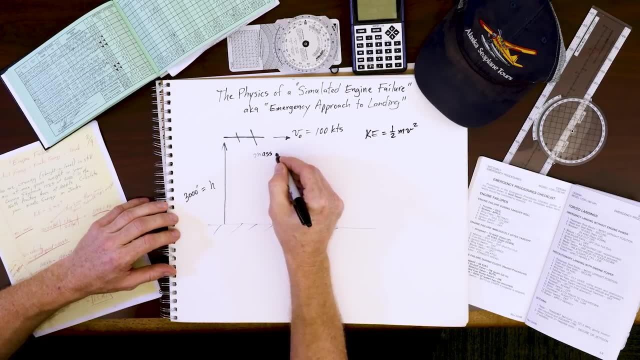 It's energy of motion. So that helps you remember. it depends on velocity here. So the first thing I'd like to do is get the mass of this airplane, Our mass m, So from our mass, we're going to get that from our weight. 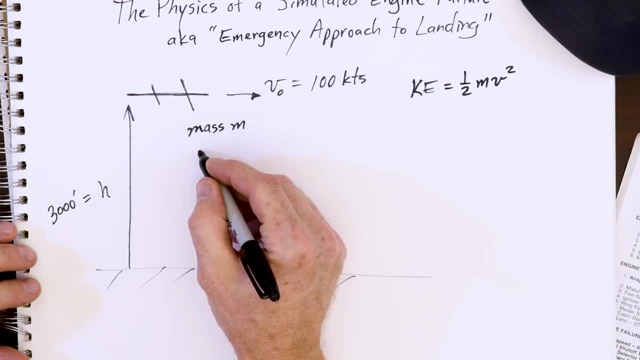 Every Riddle Private Pilot candidate knows that the max gross takeoff weight of a Cessna 172 is 2550 pounds- 2550 pounds max gross takeoff weight. They're not allowed to take off greater than that weight. So let's use that for this example. 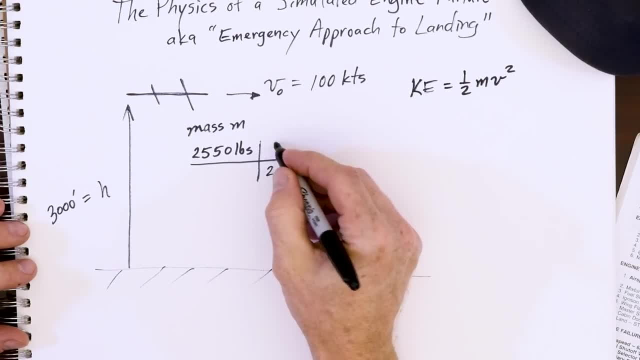 And we have a conversion that there's 2.2 pounds per 1 kilogram. In Physics class we learned how to do these conversions. We learned how to do these conversions, making sure the units cancel, And this turns out to be 1159.1 kilograms. 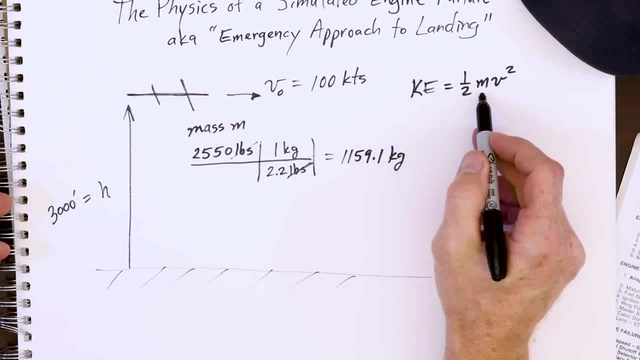 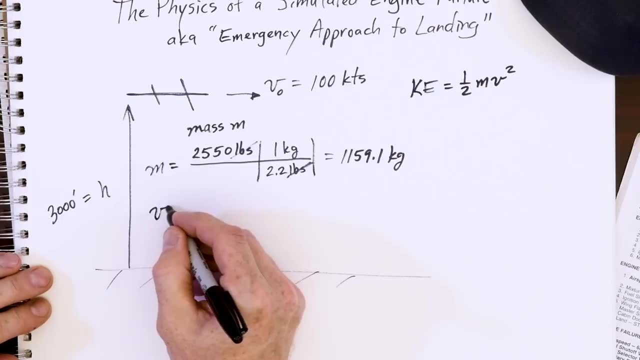 Okay, good, that's the mass. Now we need the velocity so we can get the total energy of this aircraft. Our velocity is 100 knots. So our velocity is 100 knots, Or you can write it out: K-N-O-T-S, which comes from the history of nautical sailors. 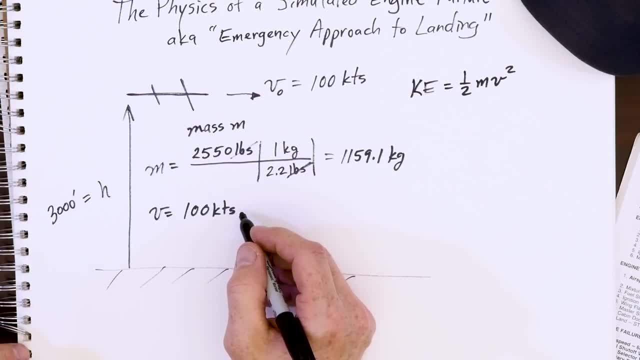 who actually threw a rope out with knots in it and counted them and used a stopwatch or an hourglass or something. For us, this means 100 nautical miles per hour, So remind yourself that knots means nautical miles per hour, just like feet per second, meters per second. 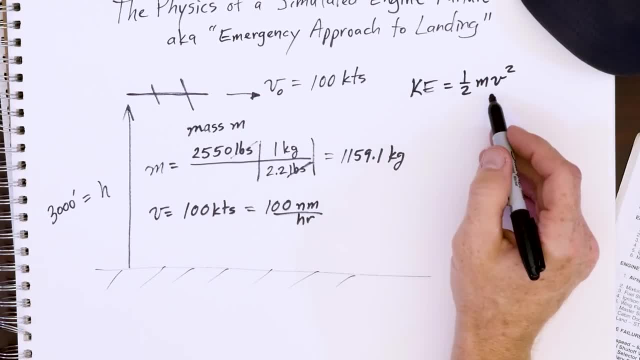 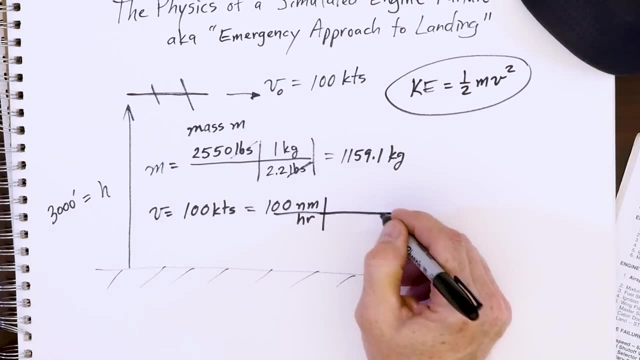 It's got to be some distance per time. So we want to convert this now into the units for Physics class and make this into meters per second. Remember, our goal here is to get the total kinetic energy for Step 1.. So we all know that a nautical mile is. 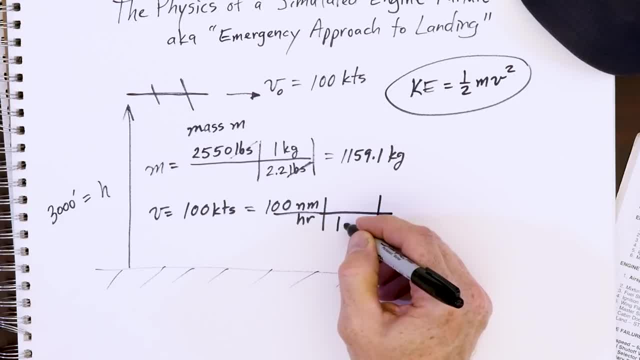 slightly longer than a statute mile. a regular mile that we're used to, And the conversion is 100 knots, is 115 miles per hour. So one nautical mile is 1.15 statute miles. Nautical miles cancel. We all know that one statute mile is 5,280 feet. 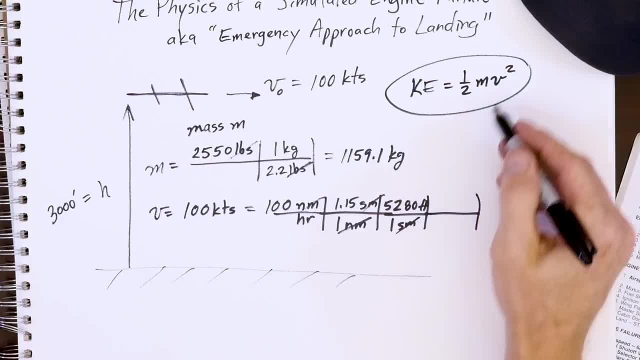 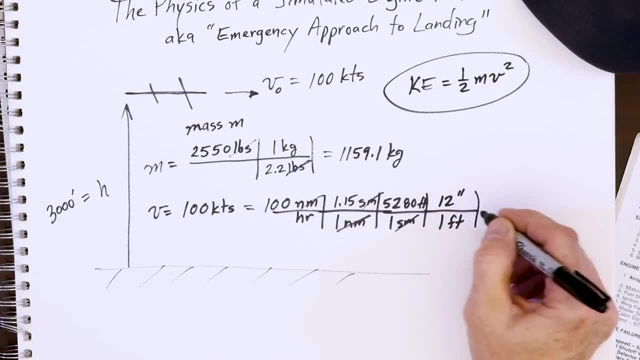 Statute miles. cancel And remember our goal is to get to meters per second. You might know of a quicker conversion. The one I know in my head is 1 foot is 12 inches And from Chemistry class I know 1 inch is 2.54 centimeters. 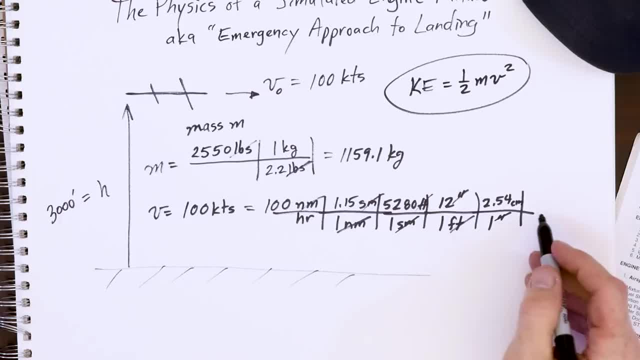 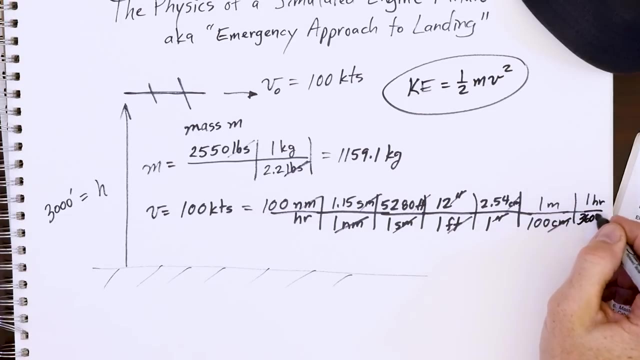 Our inches cancel. Our feet cancel. We're getting close. We now need meters. So 100 centimeters is 1 meter, Centimeters cancel. And one more step: One hour is 3,600 seconds. Why? Because there's 60 seconds in a minute, 60 minutes in an hour. 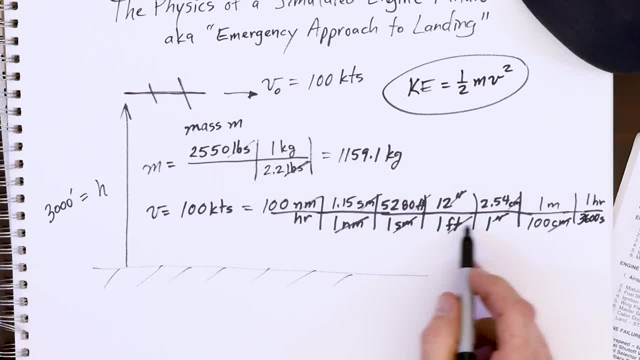 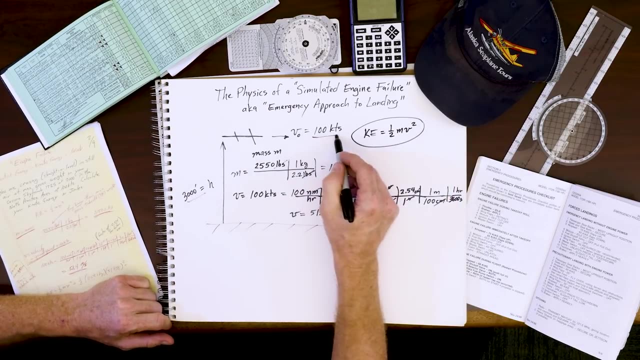 You crunch all these numbers, multiply everything on top, Divide by everything on the bottom And you end up getting velocity is 51.4 meters per second. So now we're good to go. We can calculate our total energy. We have a tremendous amount of energy at 3,000 feet and a fast 100 knots. Your flight instructor is always teaching you to dissipate that energy. Energy management control it so you don't get too slow too early. But once you've made the field and you're over your landing spot, you get as slow as possible without stalling. 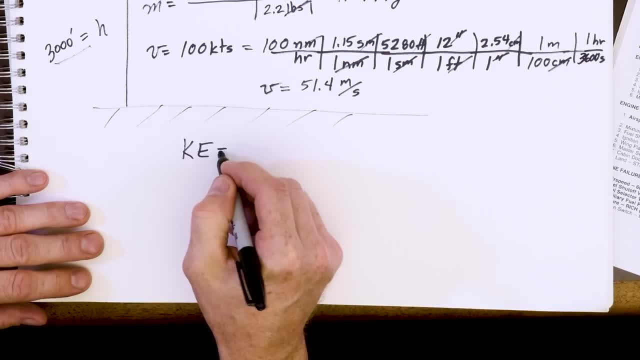 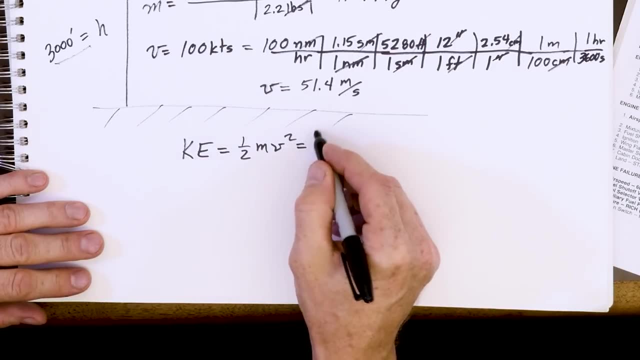 So we need to manage all this energy. So that's the first question: How much energy do we have now at 100 knots and 3,000 feet? So the first step is just the kinetic energy, mv squared. we plug in our mass: 1159.1 kilograms. 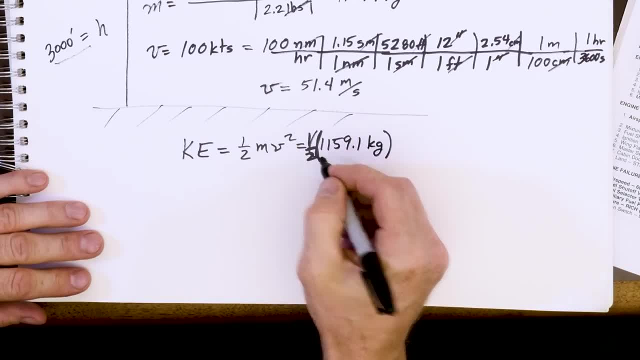 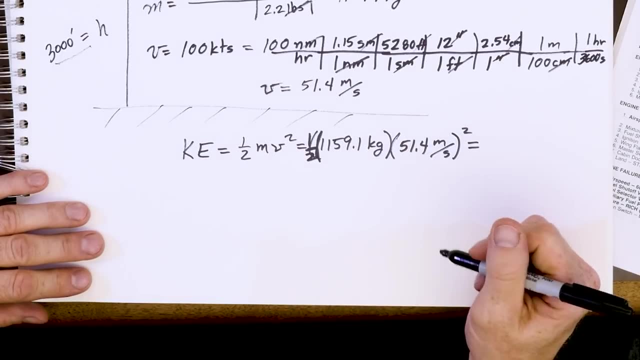 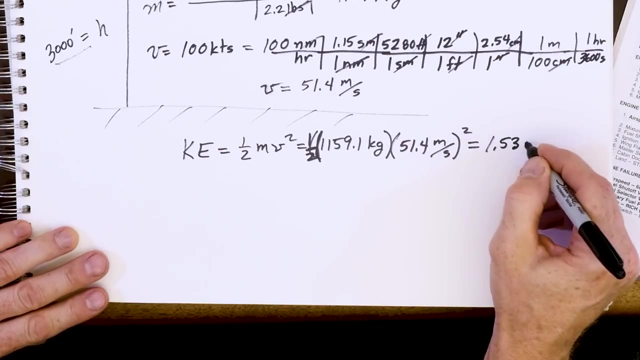 Whoops, one half. One half is in front of the parentheses Times this 51.4 meter per second quantity squared. Everyone. pause your video and crunch that in your calculator now And I will write the number down, which turns out to be 1.53 times 10 to the sixth joules. 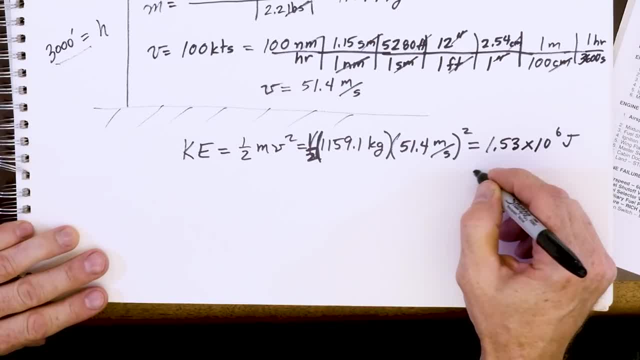 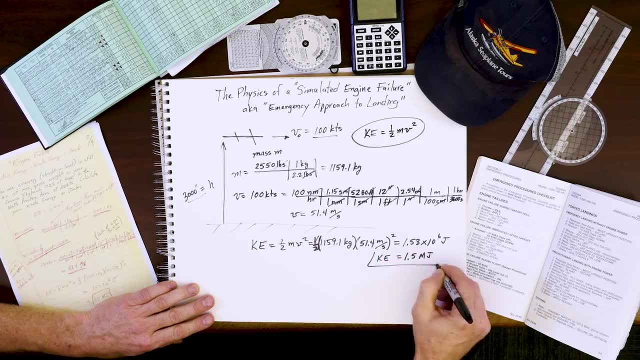 Some very large amount: 10 to the sixth is a million, And in physics class we like to be cool and call this 1.5 megajoules of energy. All right, next video clip we'll do the potential energy and the total energy.